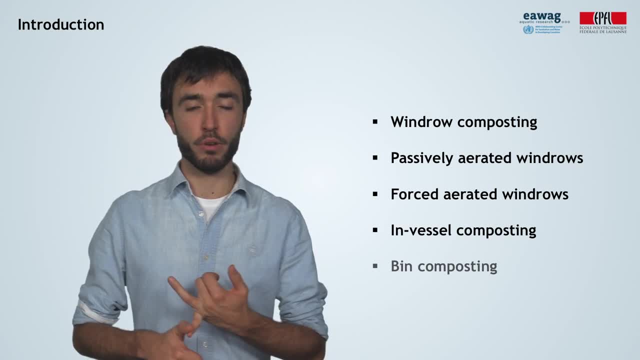 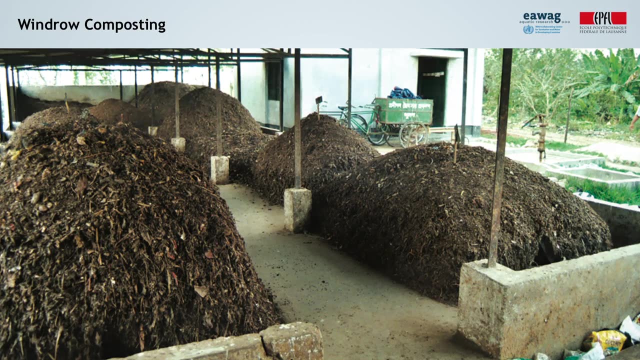 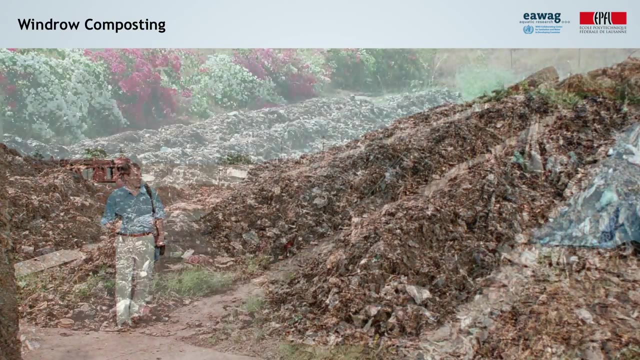 aerated windrows, in-vessel composting and bin composting. Let's start with windrow composting. Windrow is the general term for an elongated pile of stacked raw materials. This method is suited to treat large volumes of bio-waste and produce large volumes of. 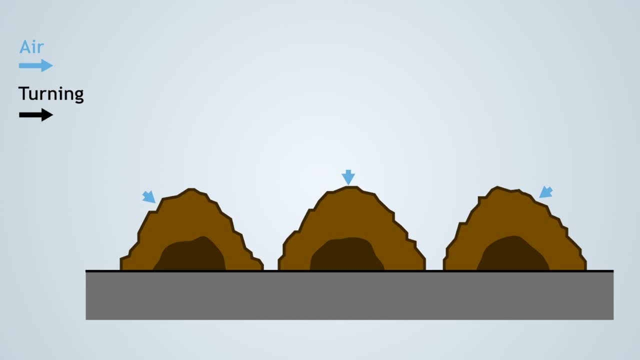 compost. Aeration of the material is crucial. Oxygen needs to be replenished as it is consumed, otherwise the piles go anaerobic in the center, following a different decomposition process and producing foul odors, Making sure that the material is porous enough for air to 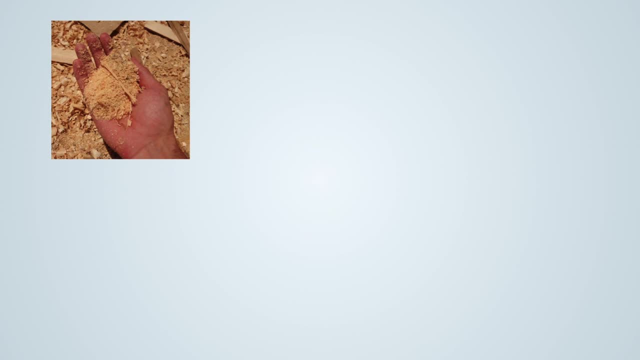 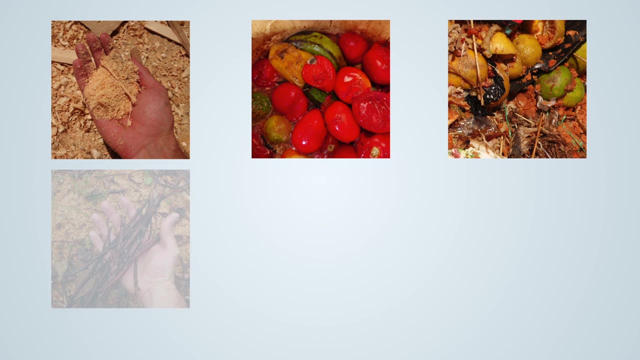 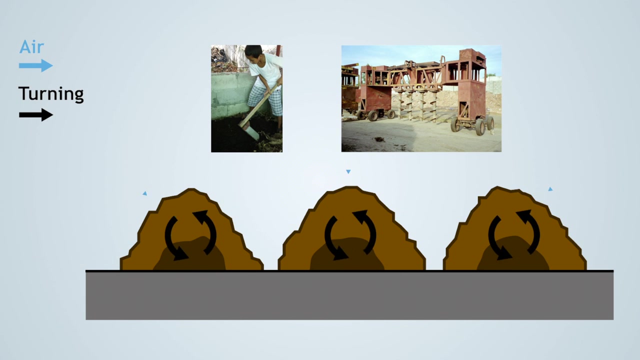 pass through is always advisable. This is achieved by mixing fine, dusty, wet or soft materials together with structure-giving materials such as small branches, cardboard or hard vegetables. In any case, the piles are normally turned, which can be done mechanically. 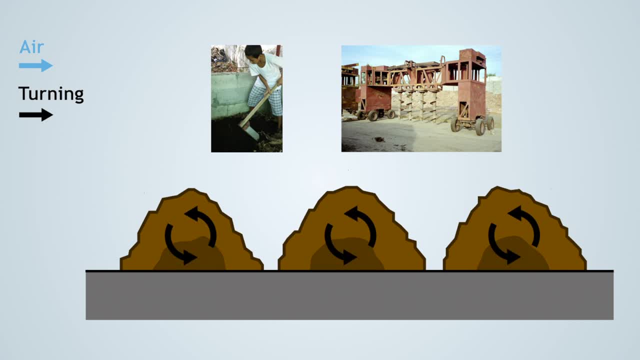 or manually. This way, the porosity is re-established and air, and therefore oxygen, get into the pile. Besides, the materials which are at the exterior of the pile can be reused. This is done by mixing fine, dusty, wet or soft. 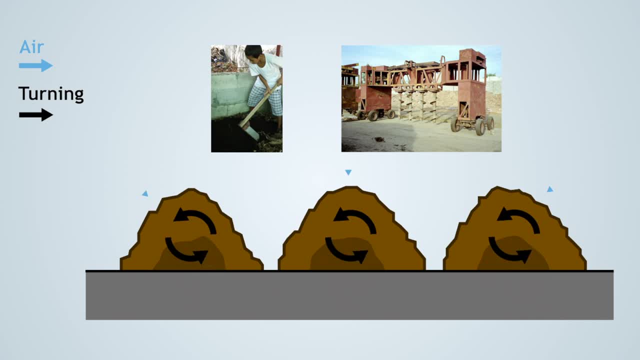 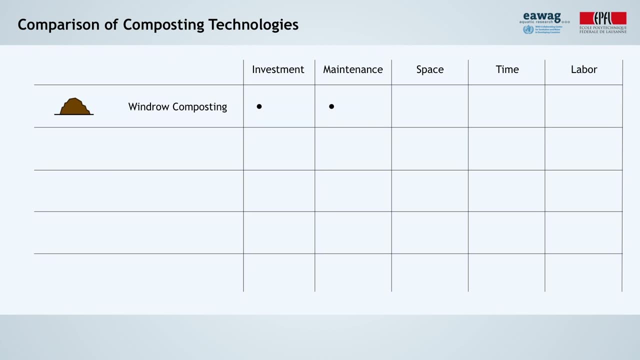 materials. The materials which are at the exterior of the pile are now in the interior so that they can be decomposed by microorganisms. This technology requires low initial investment and maintenance. However, it needs a lot of space because the windrows have sloped. 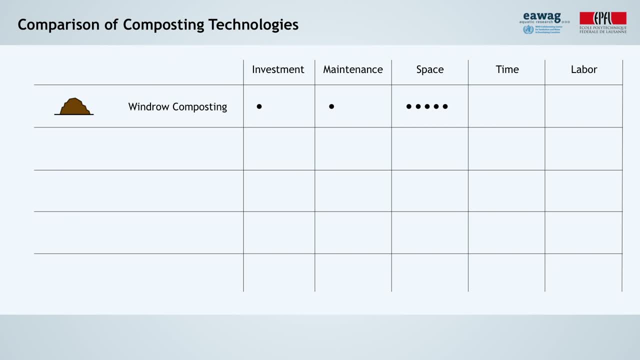 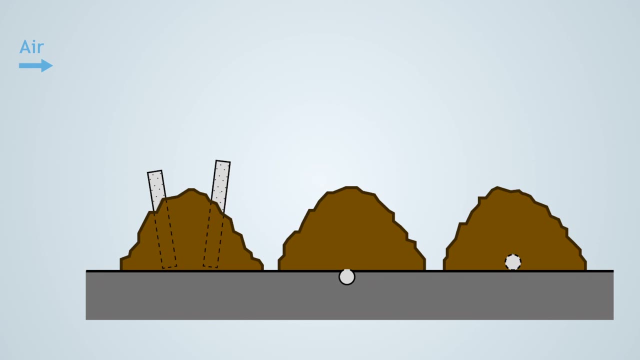 sides and cannot be put too close together. It ranks medium when it comes to the time needed for the composting process and it is labor-intensive. The second technology is passively aerated windrows. This technology consists of perforated pipes located within the bio-waste pile, which promote 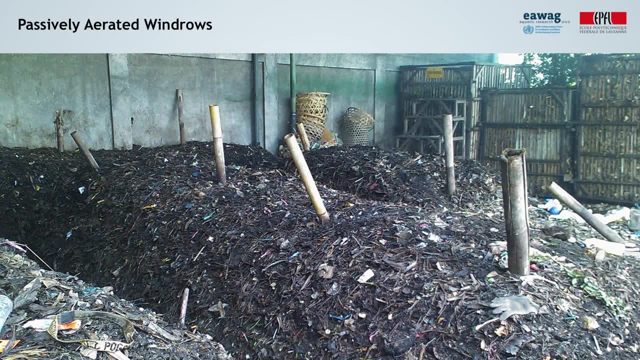 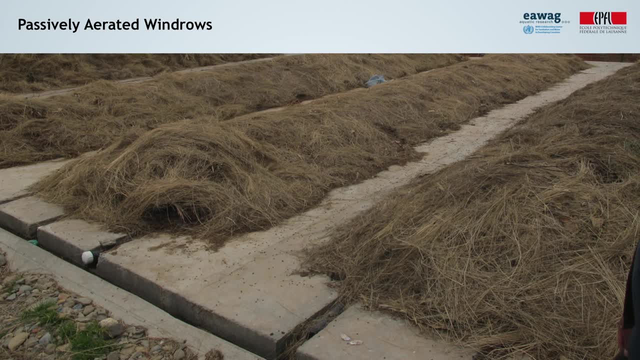 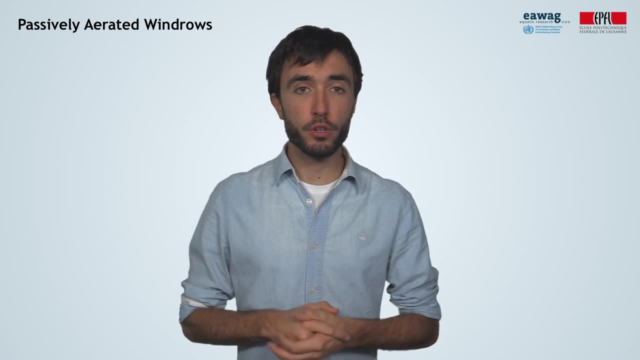 convective air flow throughout the material. The pipes can be located in different dispositions, as shown in the pictures. The air that gets into the pile brings the required oxygen by the microorganisms. These piles are normally not turned during the process. Therefore, it is important to 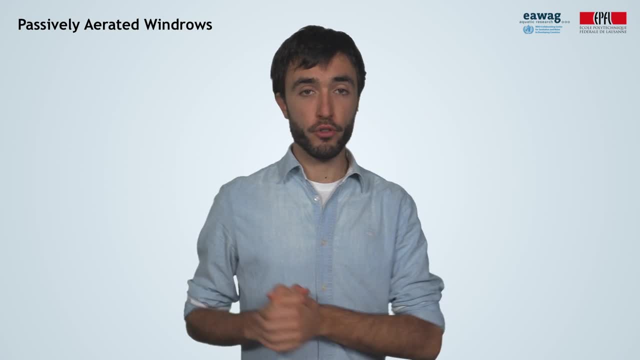 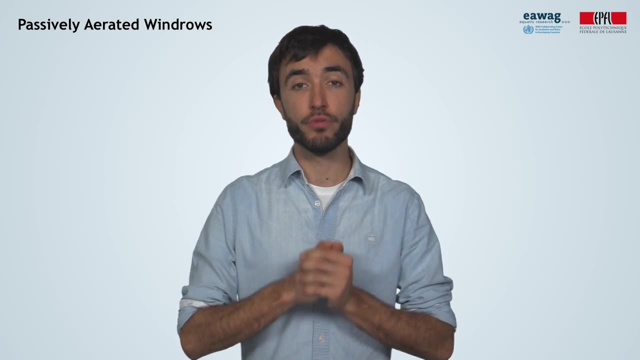 pre-mix the feedstock thoroughly before placing it on the perforated pipes. It is advisable to insulate these piles before placing them on the perforated pipes. This is done by mixing these piles with finished compost to ensure thermophilic temperatures reach the outer. 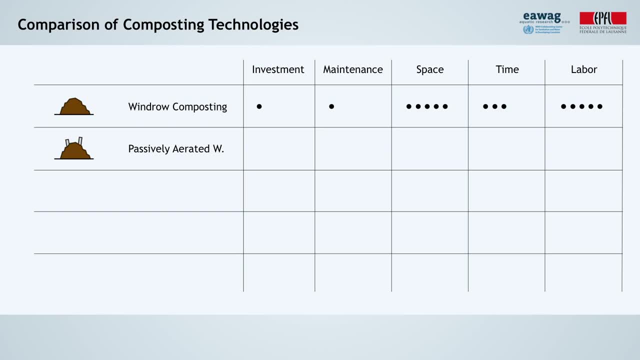 layers of the pile as well. This technology requires slightly higher initial investment and maintenance than non-aerated windrows. as it involves a passive aeration system, It has similar space requirements. the composting process might take as long or slightly shorter than with non-aerated. 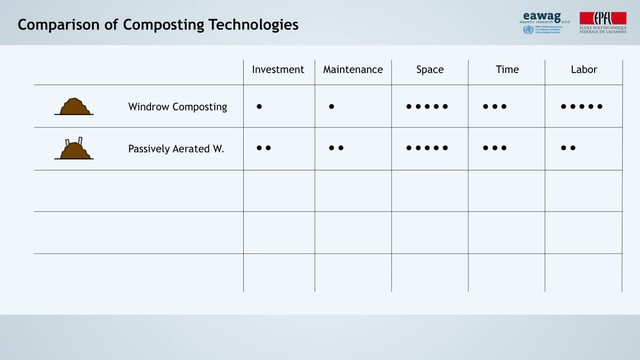 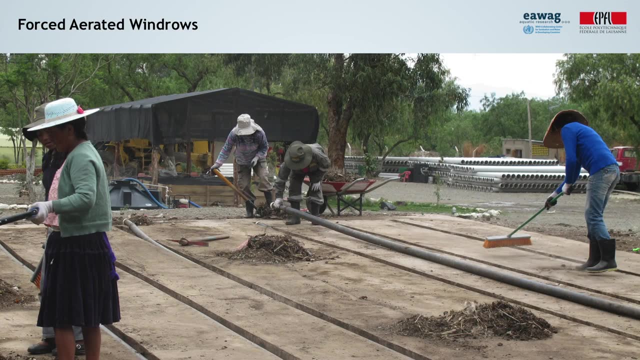 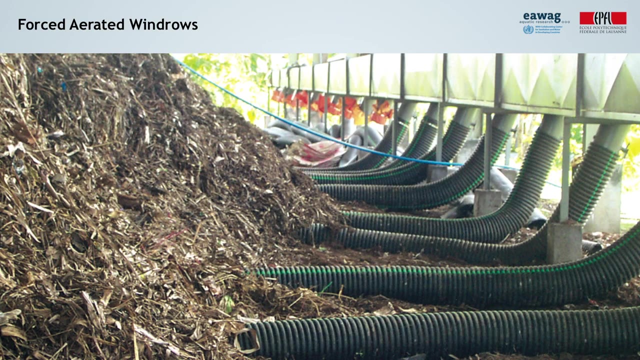 windrows, and it also requires less labor, as the piles do not need to be turned. This technology is called forced aerated windrows. They might look very similar to the previous ones. The difference is that blowers are installed at the end of perforated pipes or air ducts. These blowers inject air into the piles, preferably. 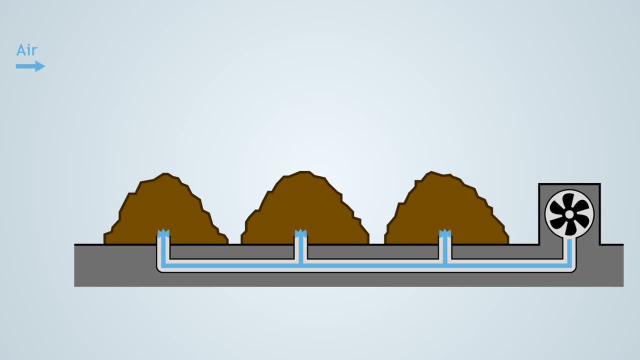 during the active phase, when the compost reaches high temperatures, Air flow can be adjusted by changing the frequency and duration of the blower. These piles do not need to be turned And, as in the previous ones, insulation with finished compost ensures that thermophilic 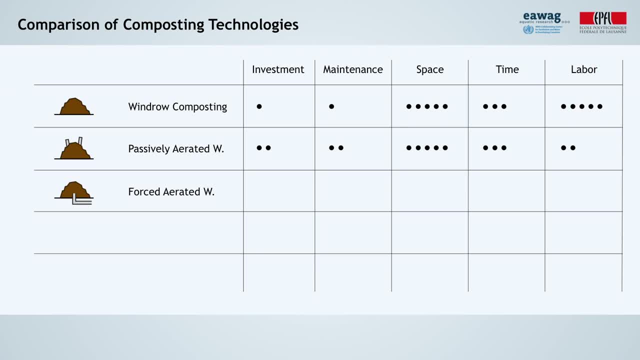 temperatures are reached in the outer layers. This technology requires even higher initial investment, given the need for a blower and aeration channels. Maintenance is also higher than the previous two. It has similar or slightly less space requirements, since the composting process is even shorter, and it requires less. 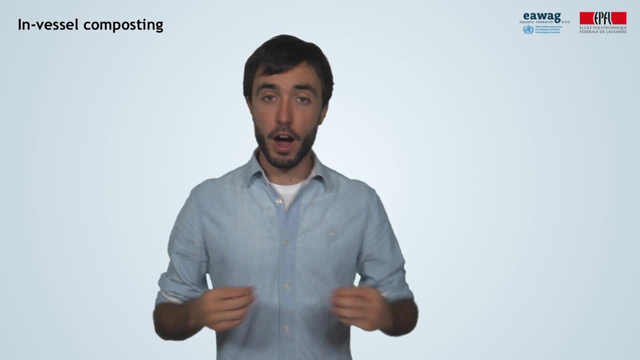 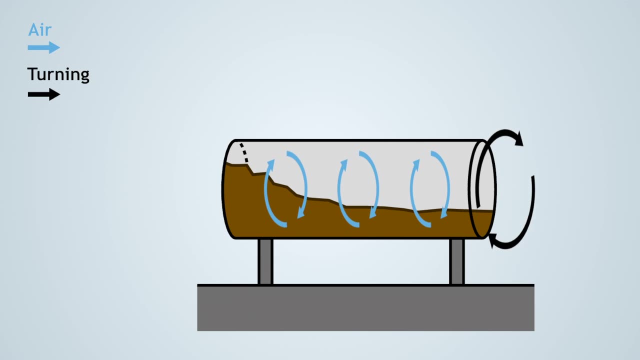 labor as the piles do not need to be turned. Our forced technology is called in-vessel composting. This describes a group of methods that confine the composting material to the outer layers of the pile. This means that the air flow can reach the inner layers of the pile and the air flow can reach the outer. 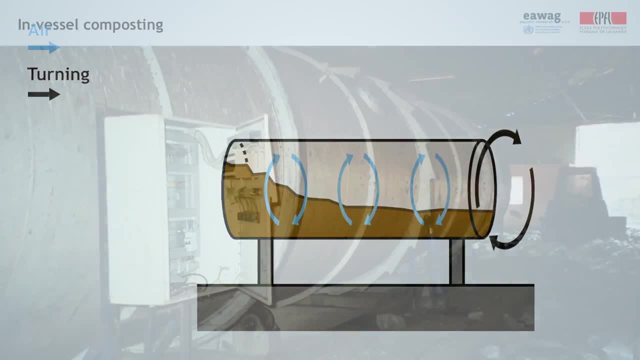 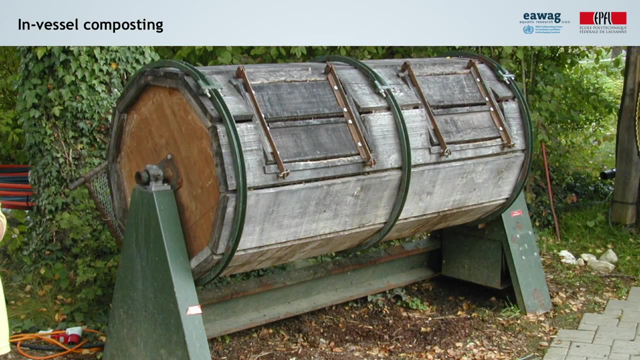 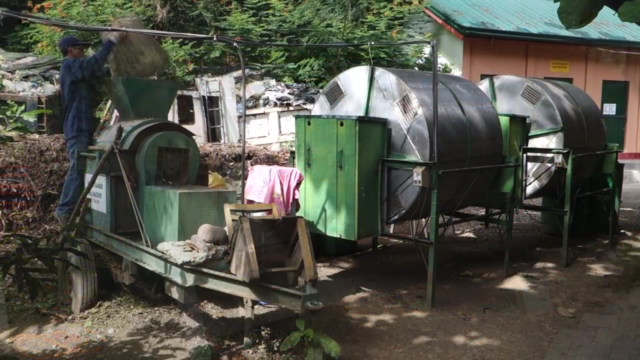 materials within a container or vessel. Installations vary from very high-tech options where parameters are monitored, acting more as a bioreactor, to very low-tech alternatives. In all configurations, air flow and temperature can be easier controlled than with other composting techniques. Turning. 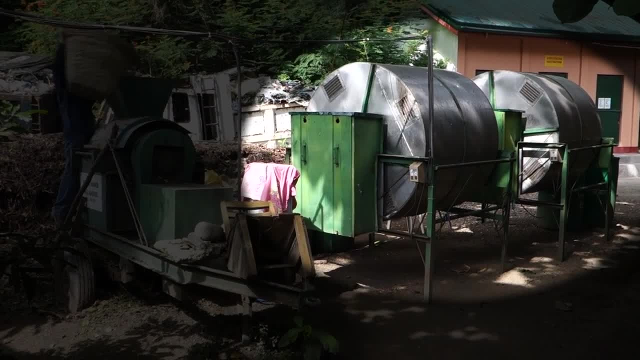 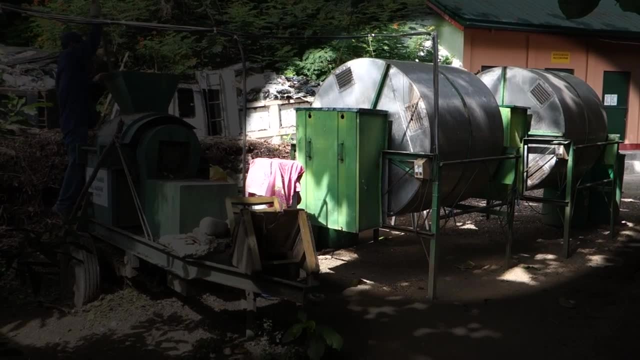 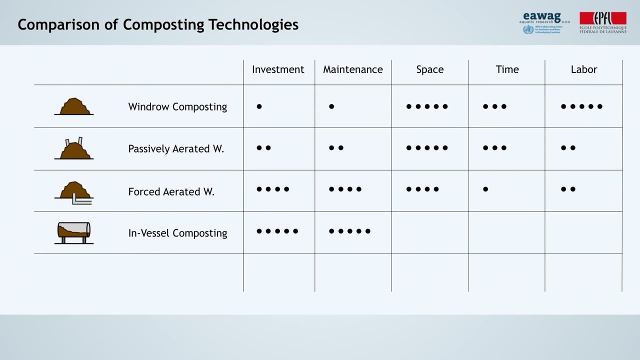 or steering takes place manually or mechanically, as seen in the video. This technology is more capital intensive and requires more maintenance than the ones seen before. It requires less surface area than with the previous technologies, since the composting process is shorter. Besides, later labor is required as the material is. 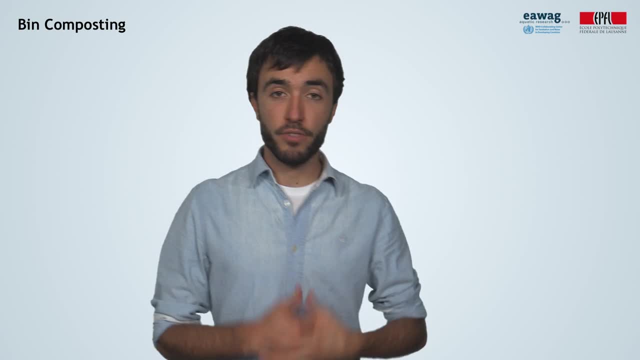 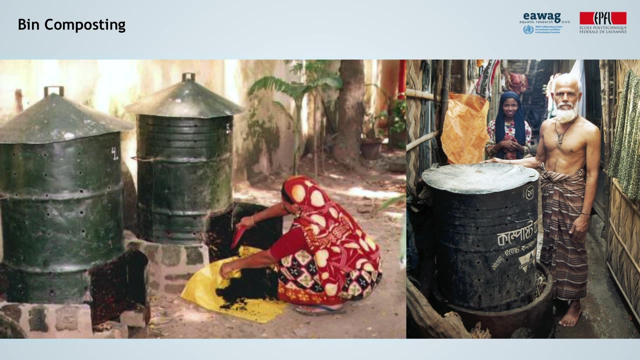 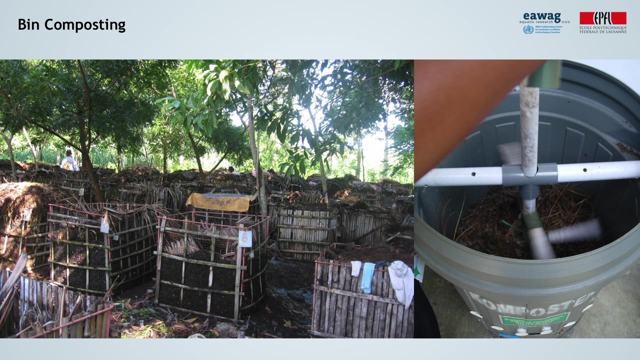 mixed within the vessel. And finally, our last technology is called bin composting. This technique is practiced mainly at household level, which will then treat little amounts of waste and produce compost for self-consumption. Biowaste is located in a container which most of the times has some sort of perforated.